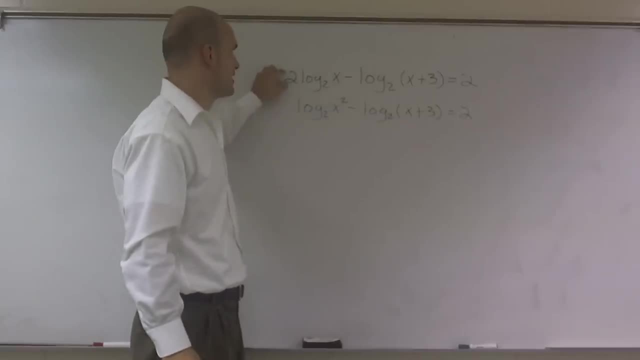 All right, that's another property of logs, that you can take your multiplier and put it back as a function. So now I'll rewrite this as log Base 2 of x squared. I'm sorry, let's change this around a little bit as x squared all over x plus 3.. 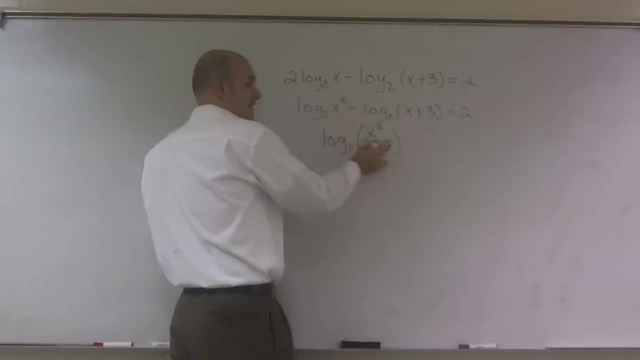 So now I'm taking the function of both of these: combined, divided equals 2.. All right, now we need to remember a couple rules. First rule is an inverse property, And what the inverse property states is: remember what a logarithm means, guys. 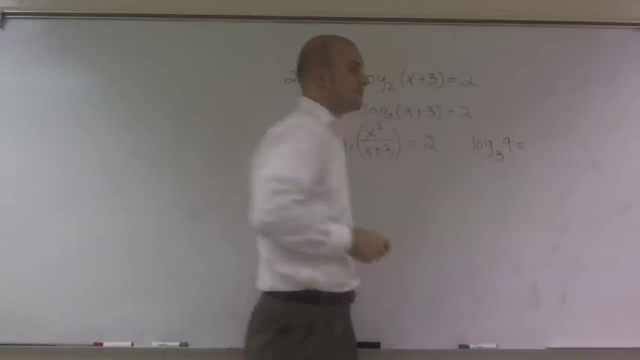 If I say logarithm of 3 to 9, that means 3 raised to what number gives you 9? And we know the answer is 2.. So if I say log of 3 raised to the third power, 3 raised to what number gives you 3?. 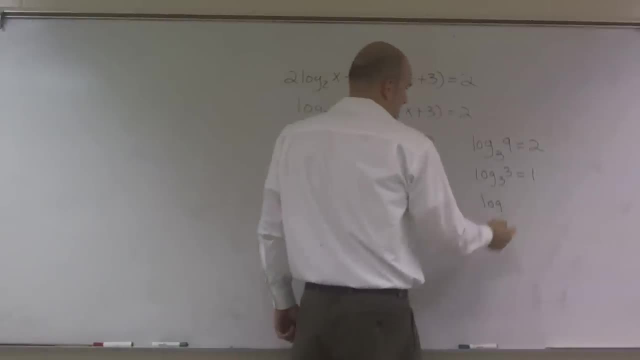 Well, the answer is 1.. So if I said log base 3 of 3 is equal to x, that answer is going to equal x. Well, why does it equal x? Well, remember, I can take that number, I can take my exponent and put it in front, as I showed you here. 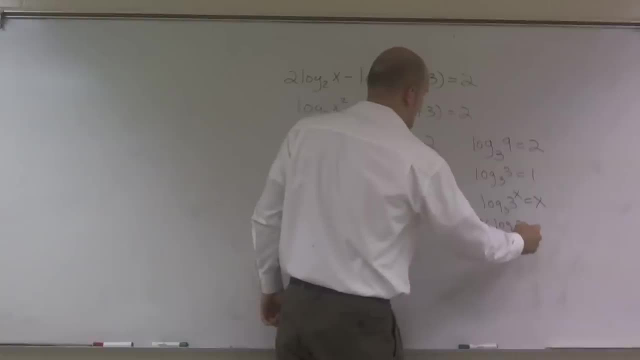 So I can really rewrite this as x. log base 3 of 3 equals. well, log base 3 of 3 is 1, 1 times x is 1,- I'm sorry- x. Okay, so this works the exact same way. 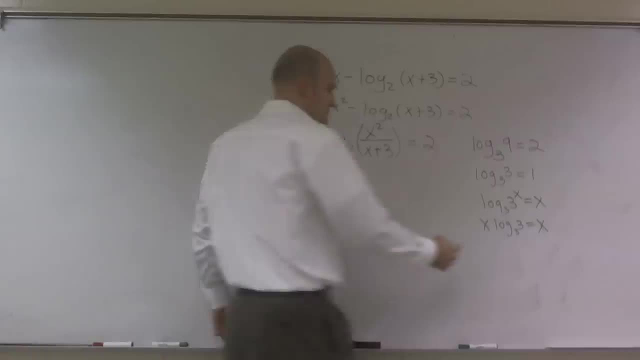 So that way, hopefully, it's easy to understand It works. the same way, if I was going to say 3 raised to the log base 3 of x, Okay, so you could say this is going to still cancel out, It's equal to x. 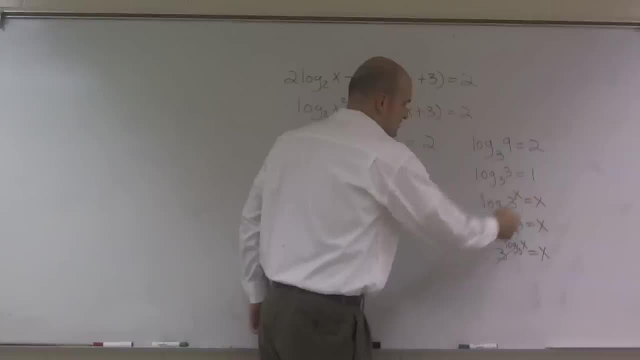 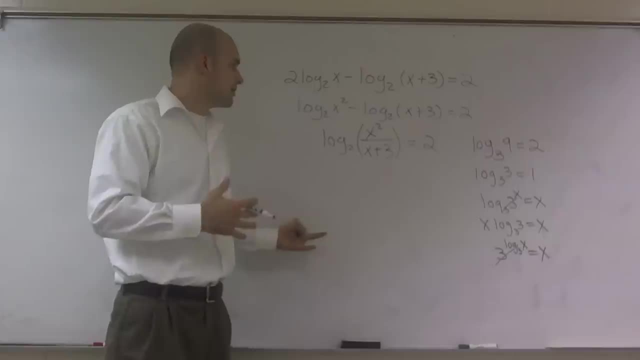 You could just rewrite it in logarithmic form or, I'm sorry, in exponential form: which 2 raised to the second power equals x squared divided by x plus 3.. Or what we could do is we could also raise, or, I'm sorry, exponentiate each side to the base 2.. 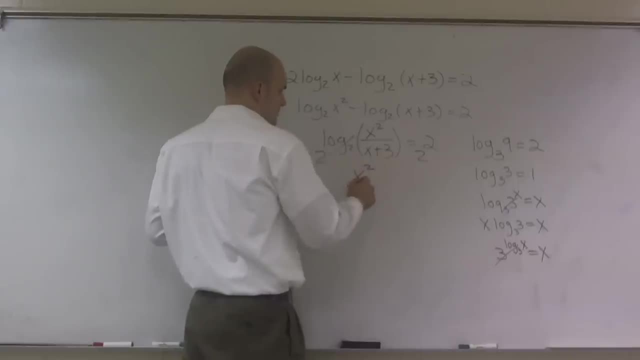 Therefore those two would cancel out and I'd be left with x squared. So I'm going to write: x squared over x plus 3 equals 2 squared. Now, if that just really confused. you just think of this this way. 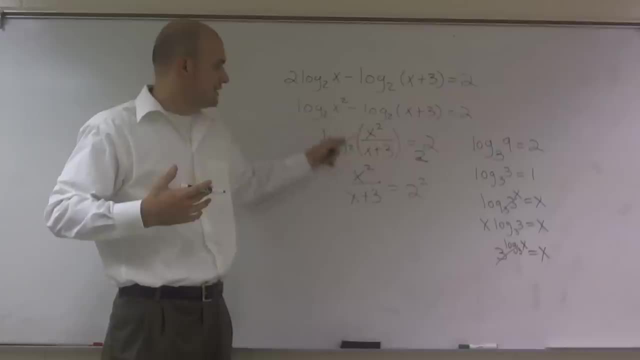 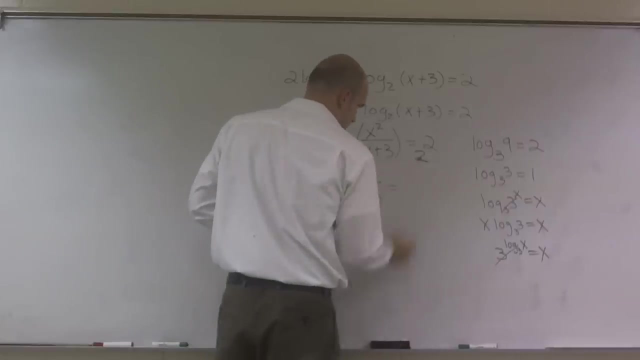 Just put it into exponential form: 2 raised to the second power equals this: okay, It's the same thing. 2 squared. I'm going to rewrite as 4 because I'm kind of running out of space. So now what we have? that's a horrible tool. 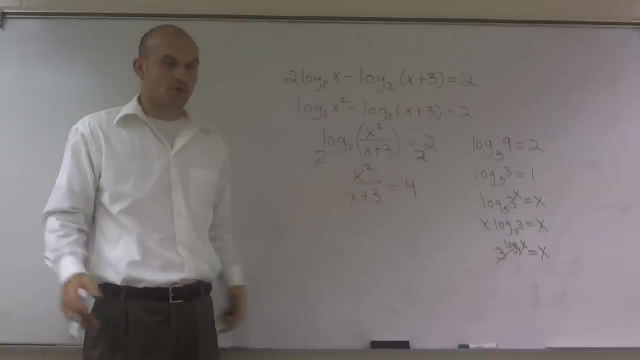 So now what we have is we have an x squared. divided by x plus 3 equals 4.. Well, I need to get rid, remember, we've got to get rid of this x, right? And one thing I notice is, since I have an x squared, I'm going to have to do some kind of factoring. 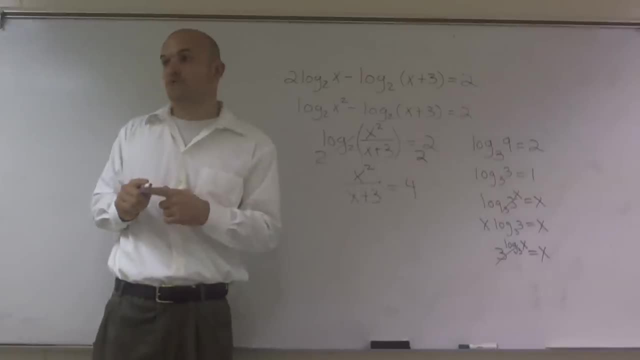 square rooting, completing the square or quadratic formula. I mean, something's going to be going on like that And since I see this other x, I'm pretty sure it's going to be a factoring or a quadratic formula problem. so, or complete the square. 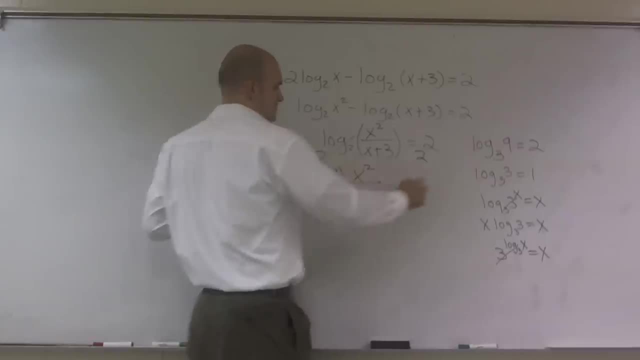 So what I need to do to get this off, I need to multiply by x plus 3 on both sides. Therefore, those will cancel out and I'm left with x squared. So x squared equals 4 times x. Let's write that a little bit better. 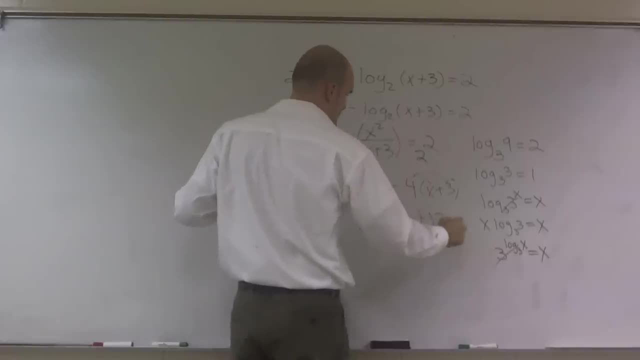 4 times x, as I do distributive property plus 12.. Then let's get them all to the same side by subtract, So x squared. let me just show you. So now let me explain why I'm having this. 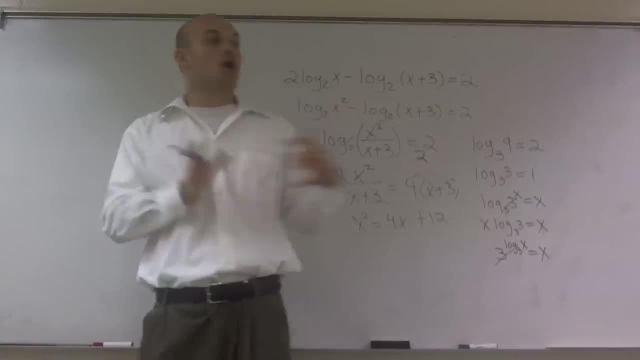 So I have x squared equals 4x plus a 12. Remember, when solving for x, you always want to get your x's all the way to the same side, right Now, when you have a quadratic, or any time you have your x's raised to a different power. 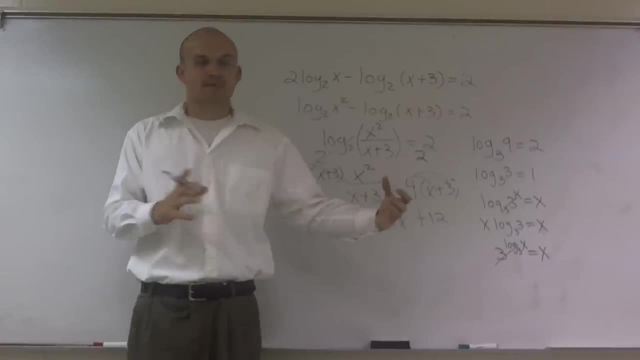 we want to see if we can set them as into linear factors, Because what I can do is I can use the zero product property rule, which states that any two numbers multiply to give you zero. one of those numbers has to be zero, So we can use that to find out factors. 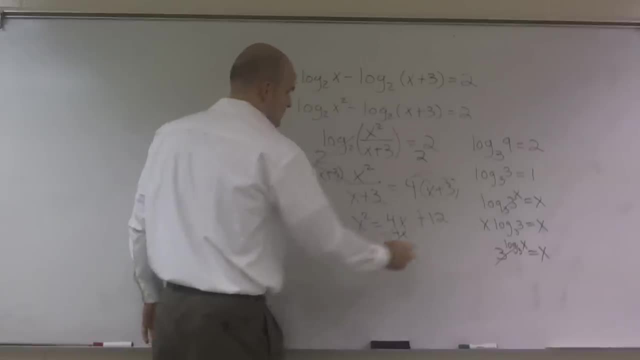 So what I'm going to do is I'm going to subtract a 4x onto both sides, Then I'm going to subtract a 12 onto both sides. So therefore I'm left with x squared minus 4x. minus 12 equals zero. 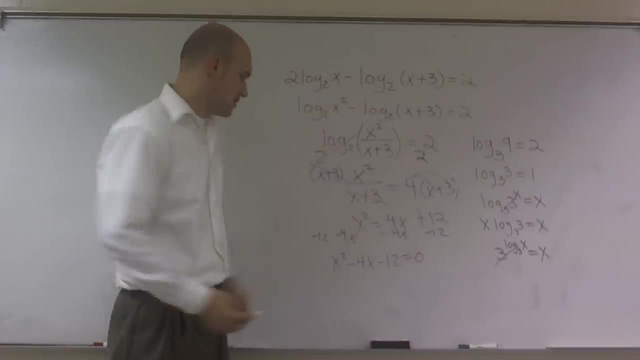 And then I say: can I factor this any further? And you say: yes, The two factors for this would be x minus 6.. So the two numbers that multiply to give you negative 12, but add to give you a negative 4.. 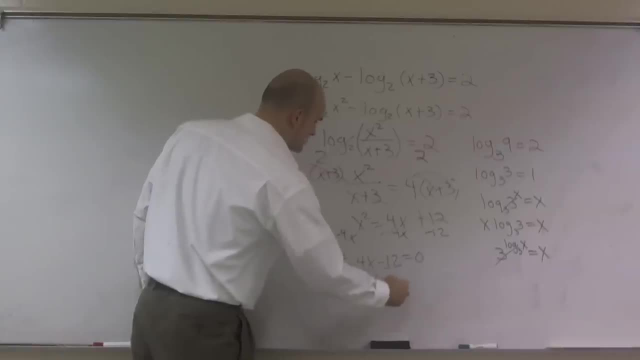 So x minus 6 and x plus 2 equals zero. So since these two numbers or these two factors multiply to give me zero, I can set them both equal to zero And say that x is equal to 6, or x is equal to. yeah, I'm sorry. 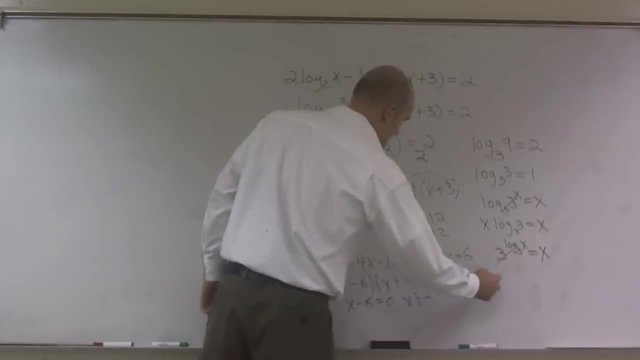 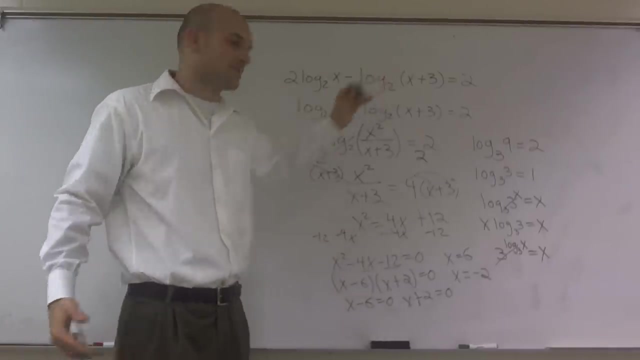 x is equal to 6, or x is equal to a negative 2.. Now, those are my two possible solutions, But what I'm going to do is I'm going to plug them back into my logarithm and see if they both work. 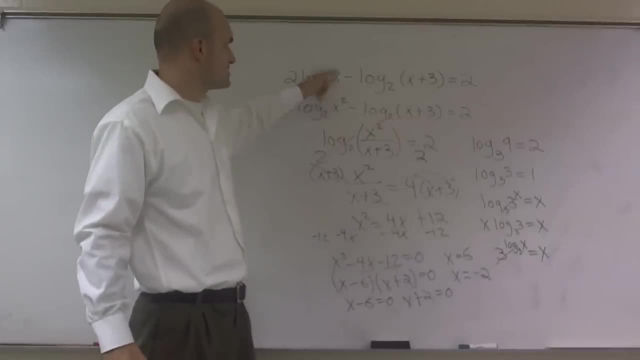 So I plug 6.. So if I take log base of 6, that's going to work. However, if I take log base of 6 plus 3, that's going to give me 9.. That one does not work. 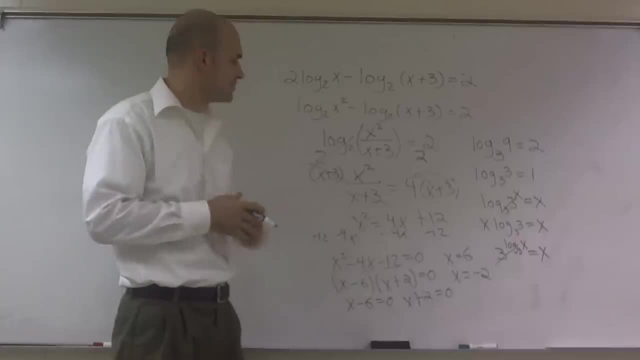 Then I go ahead and take a look at this problem and I say x equals a negative 2.. Well, if I plug in x equals negative 2 in for there and for this function, I can't evaluate: x equals a negative 2.. 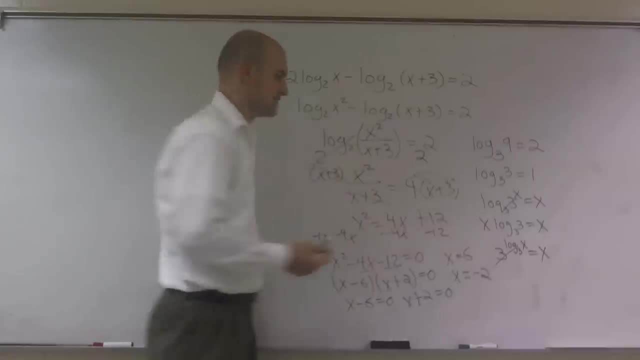 So therefore that one is not going to work because you can't take the logarithm of a negative number Okay. So therefore that will not work. But if I put a negative 2 for there it would work. 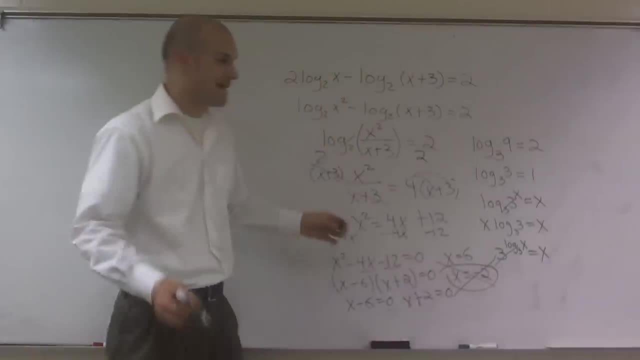 But anyways, that is an extraneous solution. It does not work. So x equals 6 is your only solution. Thank you.